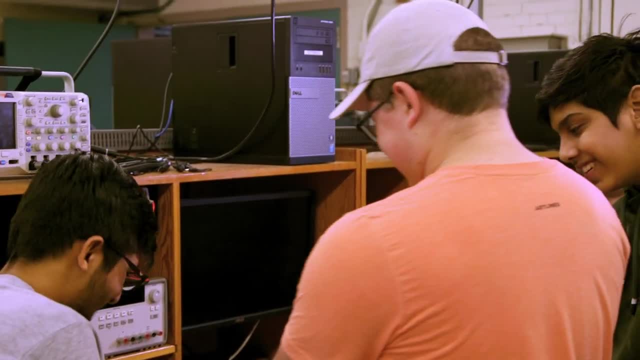 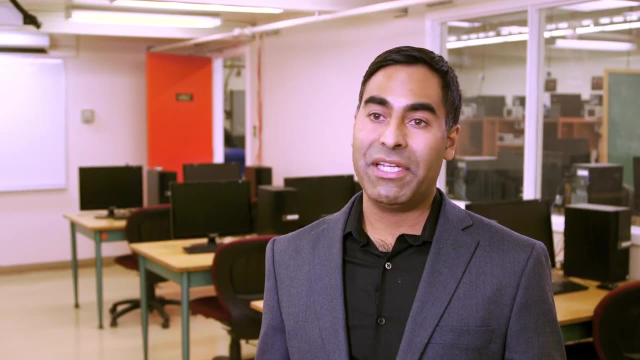 in and I have not regretted it one time. You know some assignments might be hard and stuff, but overall, like it's, it's really good course. everyone's really nice, the teachers are nice. you have the lab here. you get to apply things You know. leading-edge program that offers. 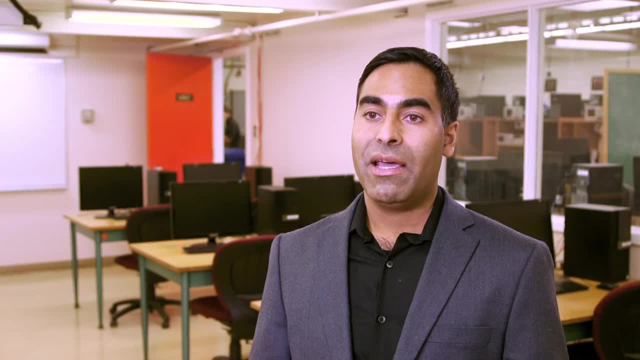 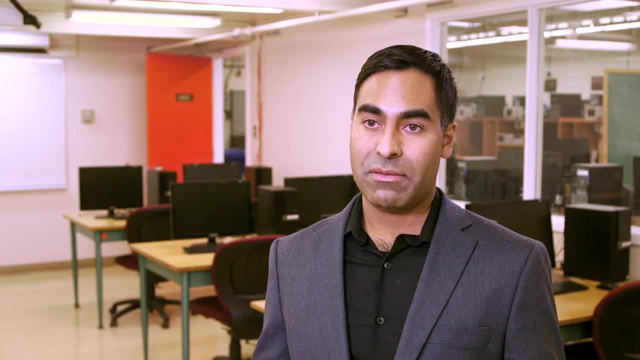 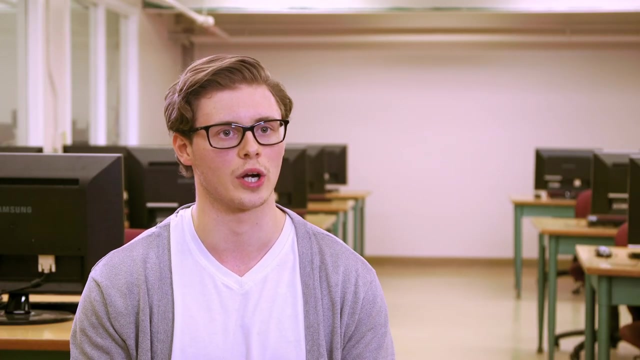 content that is the demand of industry and it's also nationally accredited program. We also have a cooperative education program that's integrated. 33% of your time in this course is you're on. you're actually out in the industry working. You get to make money and you get to work. 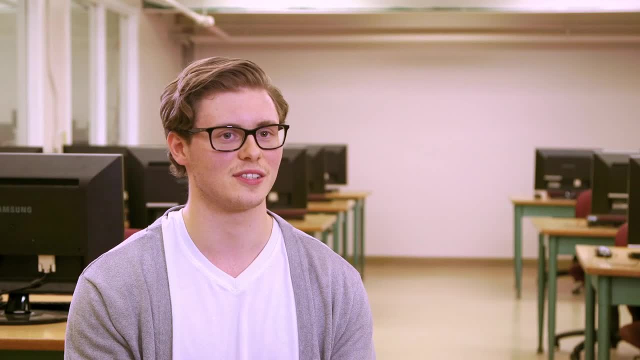 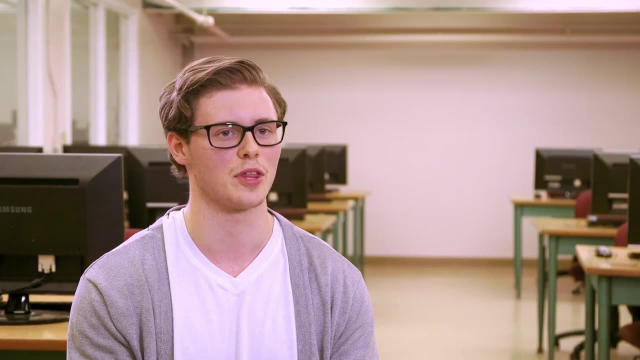 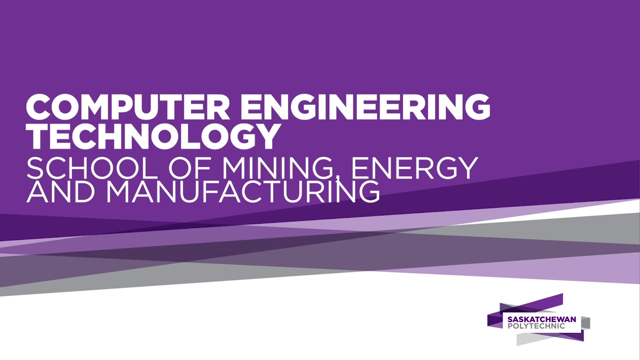 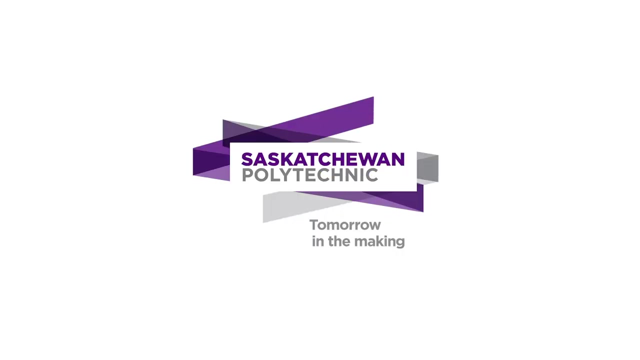 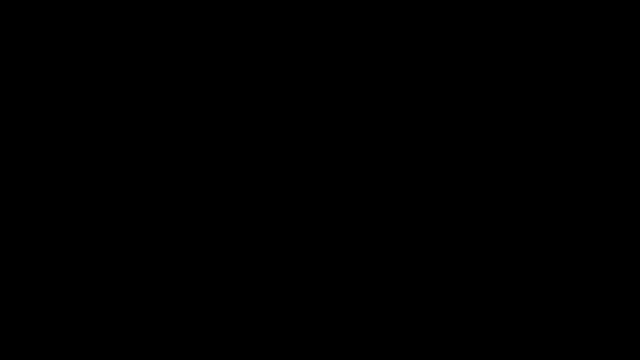 You get to learn stuff. Technology industry is great. it's guaranteed jobs for people. it's future-proof. you're able to find positions very easily with the technical skills that you get from this program. you.